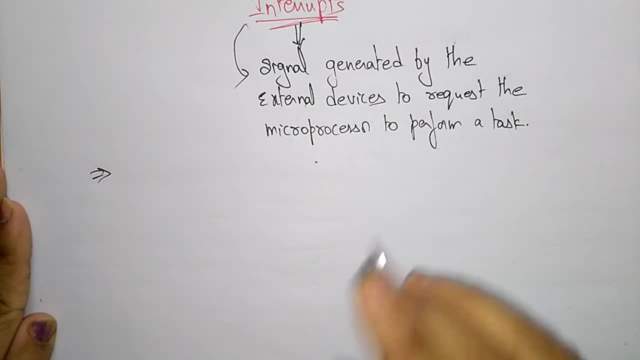 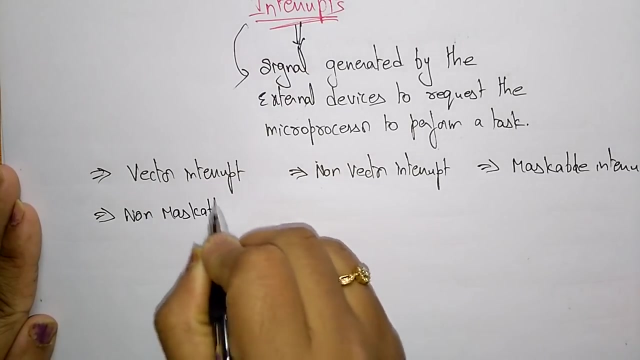 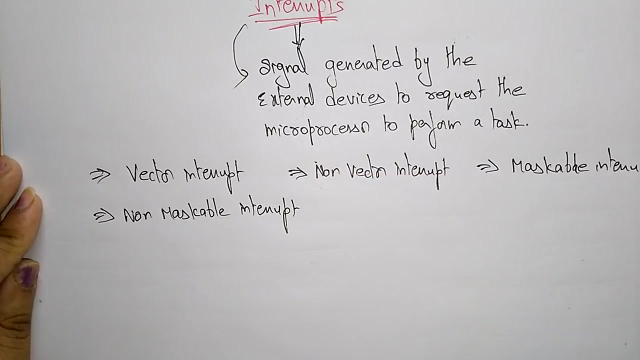 a groups based on their parameters. so the different interrupts that are present in the 8085 microprocessor, or means a processor that accepts the interrupts, or vector interrupt, next non-vector interrupt, maskable interrupt and non-maskable interrupt. so these are the four different interrupts that are classified into groups based on their. 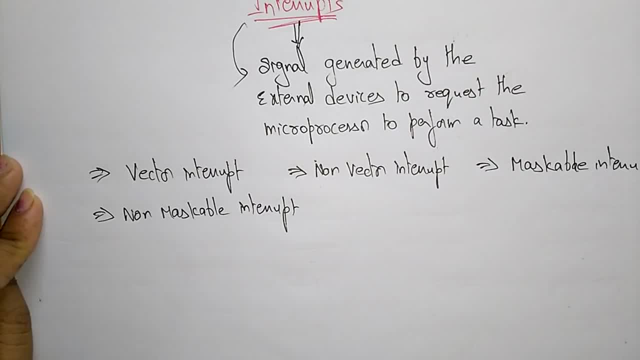 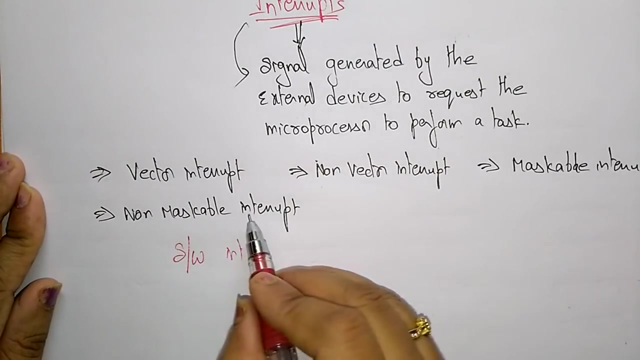 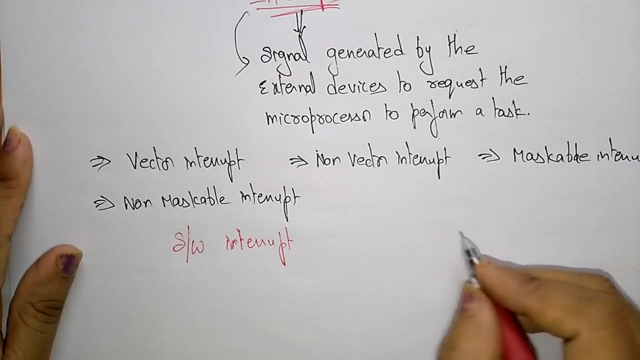 parameters. so actually, 8085 microprocessor. it accepts the interrupts and those interrupts are divided into two. mainly one is the software interrupt. so before going to know about these interrupts, let us see the two different interrupts that are present in that accept by the 8085 microprocessor. 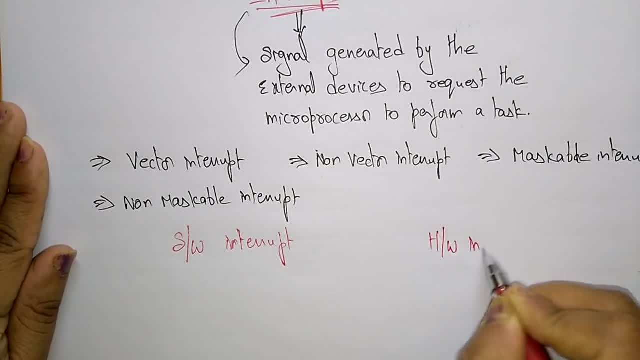 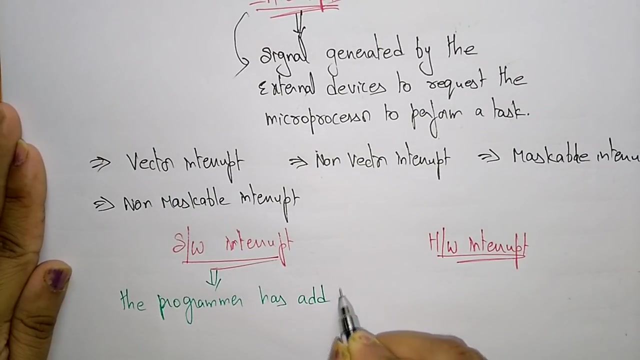 software interrupt and hardware interrupt. so what is the software interrupt and what is the hardware interrupt in software interrupts? so this type of interrupt the programmer has the programmer has not specified until then, is it adequate? it is adequate if it is given to the controller, Click 3834 to turn on the software. 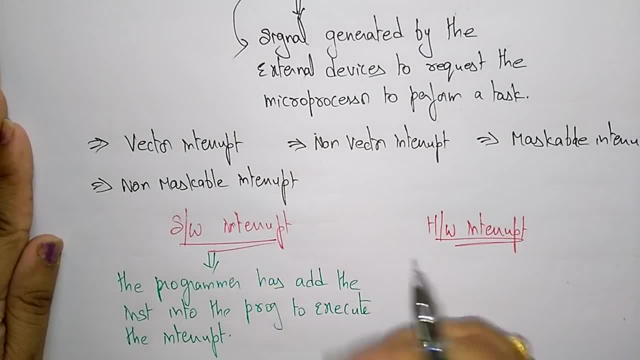 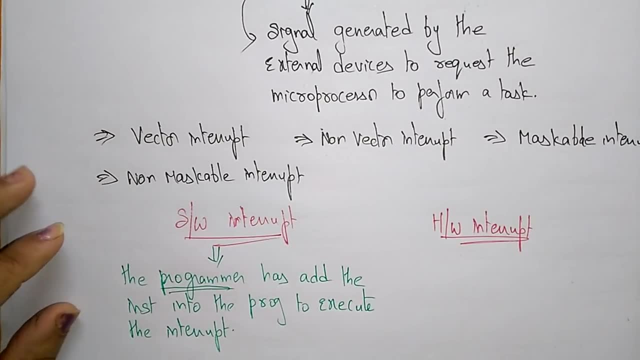 ah, now to see these two types of interrupt here. we need to create a program here. so first let us open this program- we will call it software interrupts- and want to use this program to create this program. so I 드� personn 하고 seconds given so we can say that we have the program. 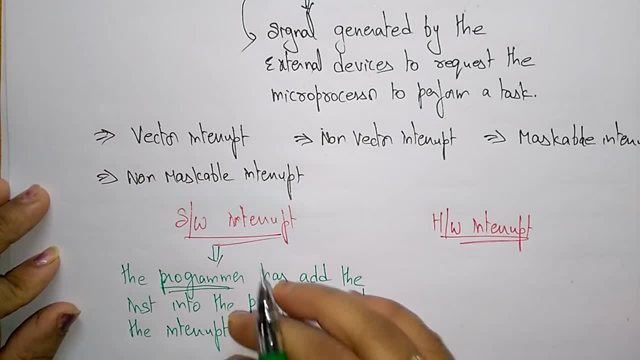 type: andnow we will add the instructions into the program to execute the interrupt. to execute the interrupt. to execute the interrupt, so that you call it as a software interrupt. what is that software? write some instruction in the program to execute this interrupts, so those you call it as a software. 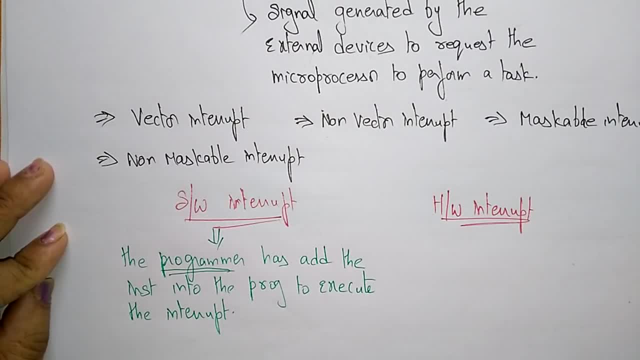 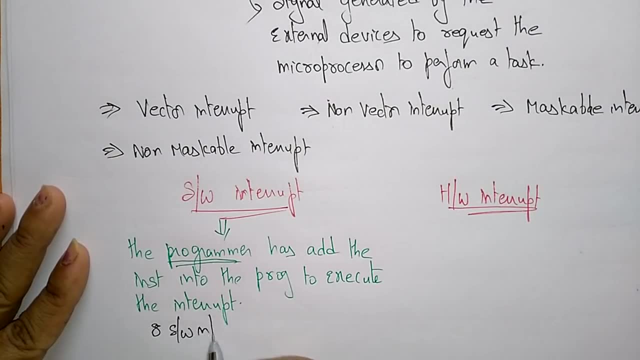 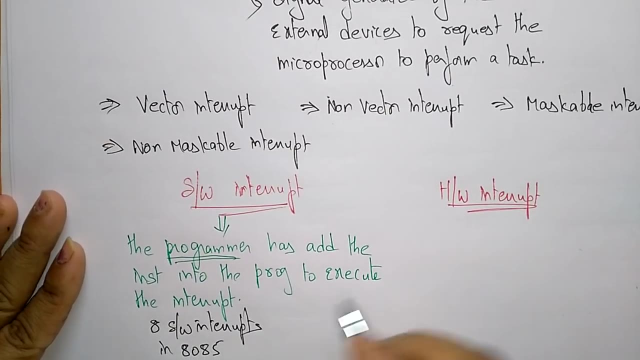 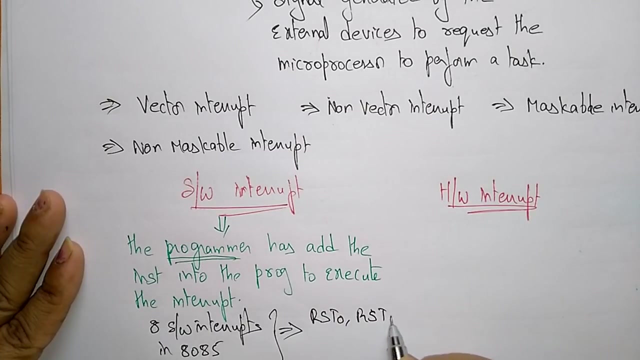 interrupts. so there are total eight software interrupts that are present in 8085 microprocessor. so those eight software interrupts are eight software interrupts are present in 8085 processor. so those eight software interrupts are: rst0, rst1, rst2, rst3, rst4, rst5, rst6 and rst7. 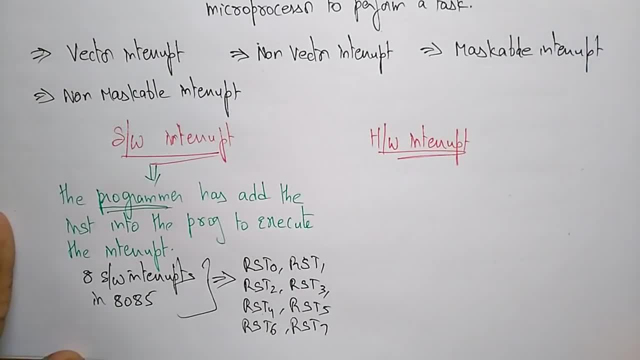 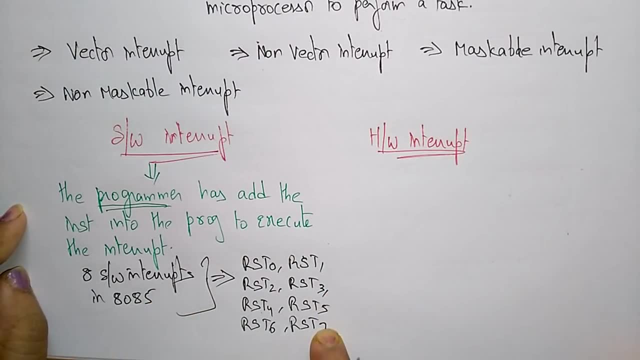 so these are the four software interrupts that are accepted by the processor. so those eight software interrupts are rst0, rst1, rst2, rst3, rst4, rst5, rst7, by the 8085 microprocessor. so these you call it as a software interrupts in 8085 software interrupts. 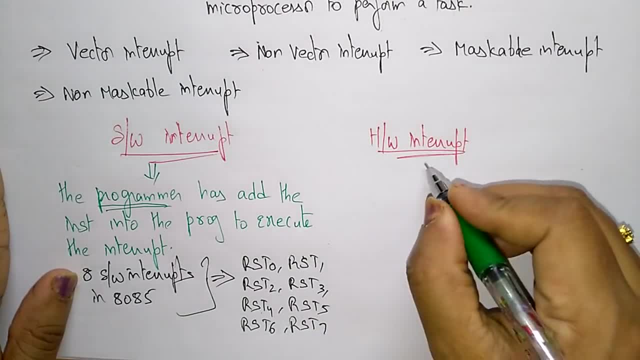 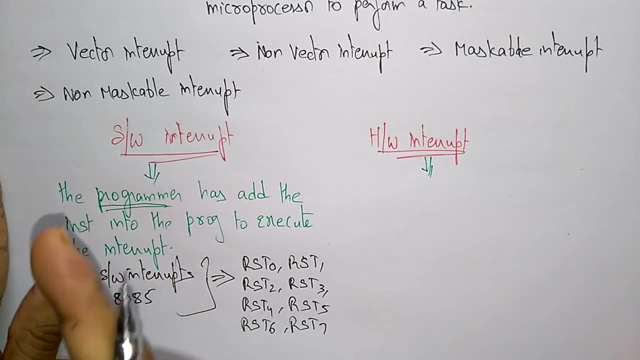 now let us see what is a hardware interrupt. hardware interrupt means it is the interrupt that caused by the hardware. so this is software means the programmer is going to be add some instructions to the program to execute the interrupt, whereas hardware interrupt is the interpreter caused by the uh, by the hardware devices, some external devices. so these are 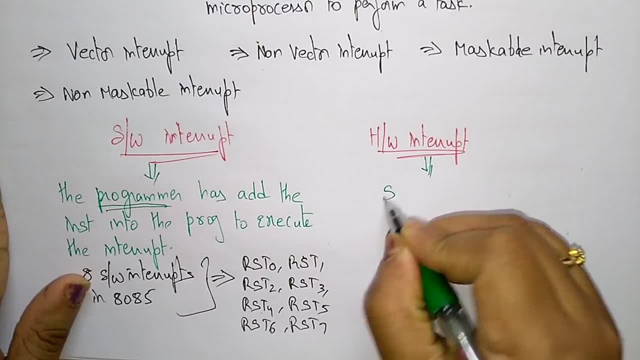 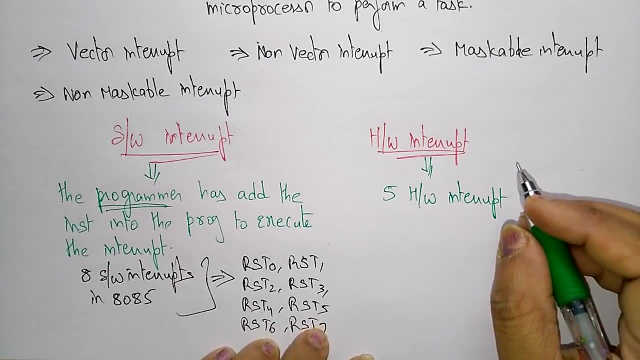 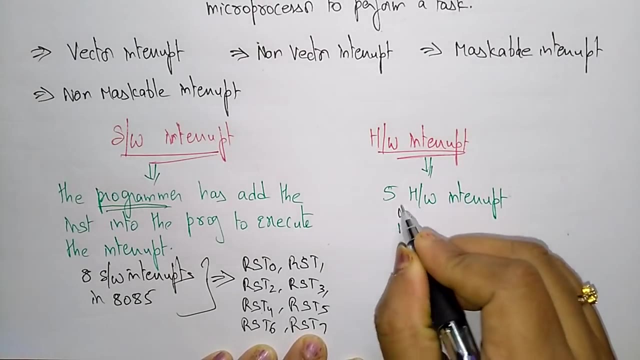 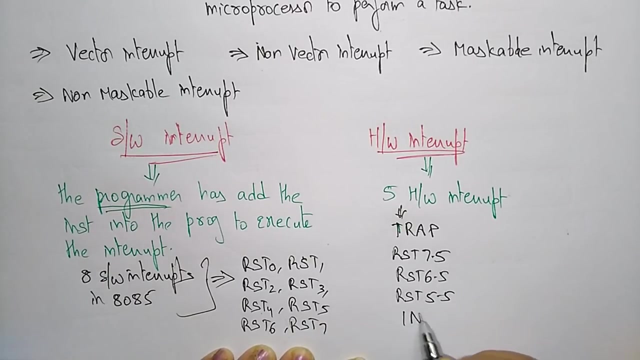 these hardware interrupts, or, uh, totally five hardware interrupts- are present in 8085 microprocessor, so the pins that are connected to this hardware interrupts are trap. the five hardware interrupts are trap: rst, 7.5, rst 6.5, rst 5.5 and intr. so these are the five hardware interrupts, five hardware interrupts and 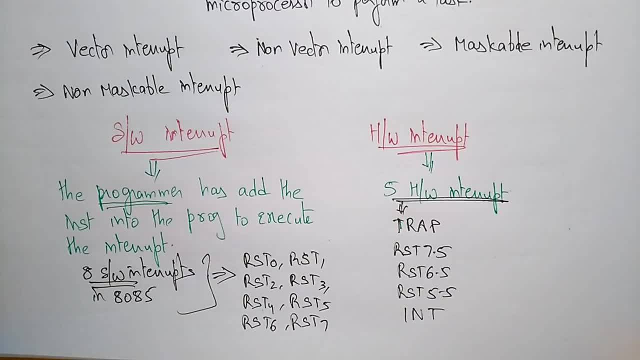 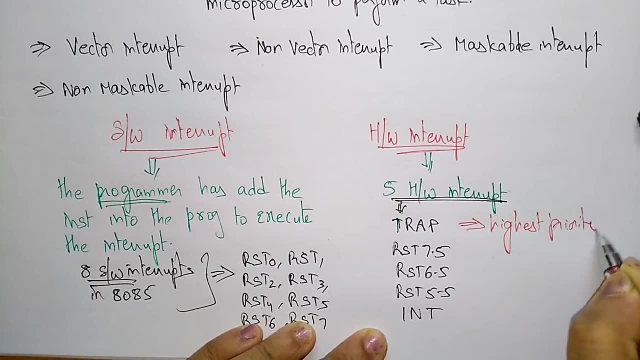 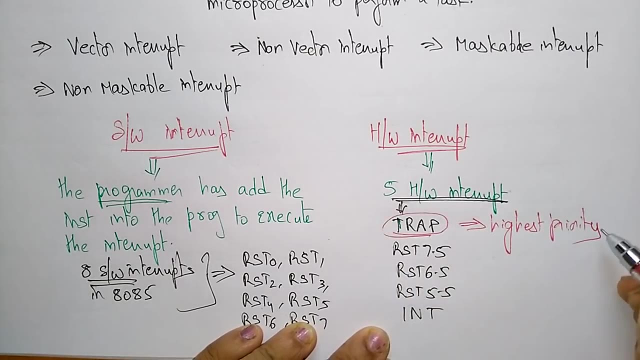 eight software interrupts. so these here the trap is having the highest priority. so whenever the trap interrupt is occurred in the program means in the while executing the programs, whenever the trap signal is activated. so this request has to be served first. once the trap signal service request is over, it can the process continues within the previous instructions. 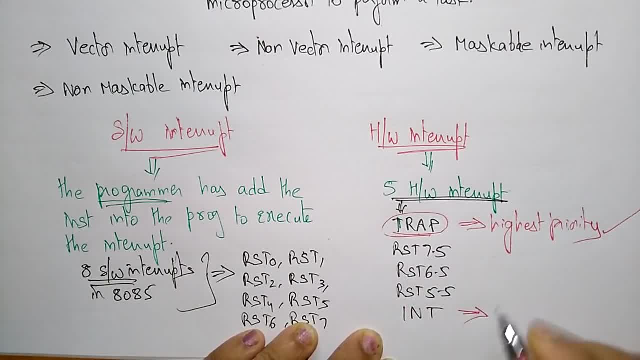 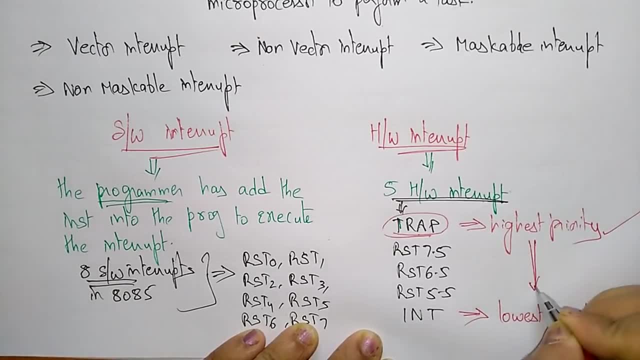 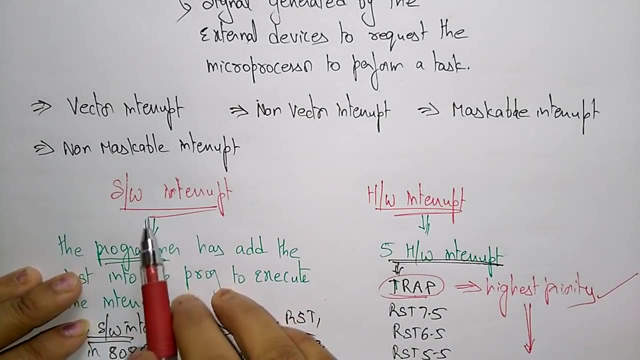 so this trap is having the highest priority and int is having the lowest priority. the priority will be decreasing from here, like this. okay, so these are the two different interrupts that are present in the uh 8085 microprocessor: software interrupt and hardware limit. now let us see what is the 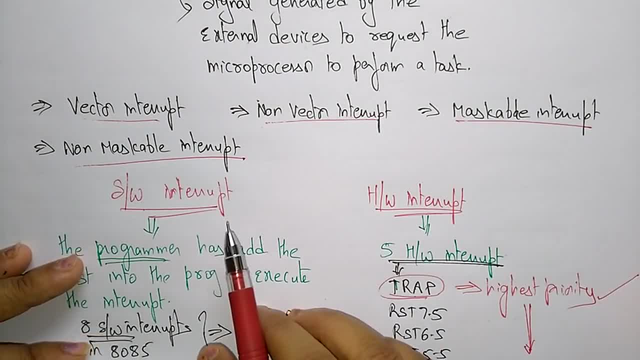 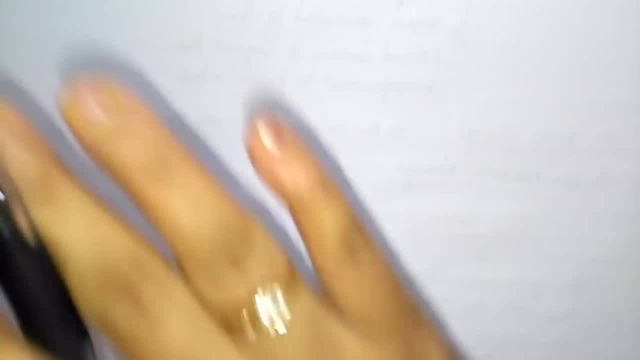 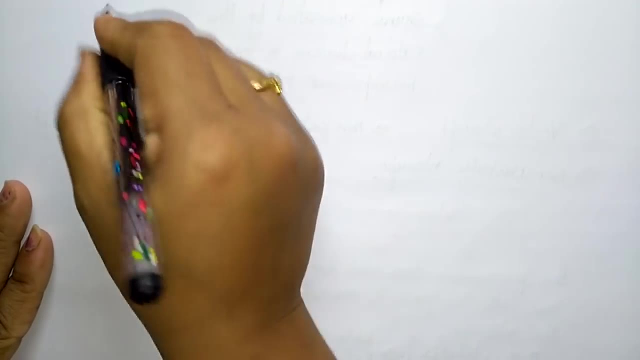 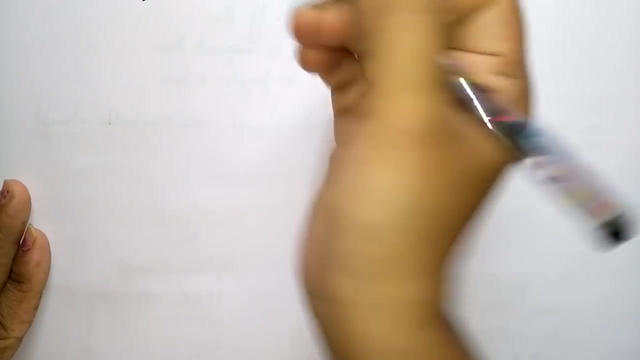 vector interrupt, non-vector, maskable and non-maskable interrupts, if you like that. so these interrupts are classified mainly based on their parameters. so the parameters that are used, based on the parameters, these interrupts will be generated. vector interrupt. so vector interrupt means here: uh, interrupt address is known to processor. 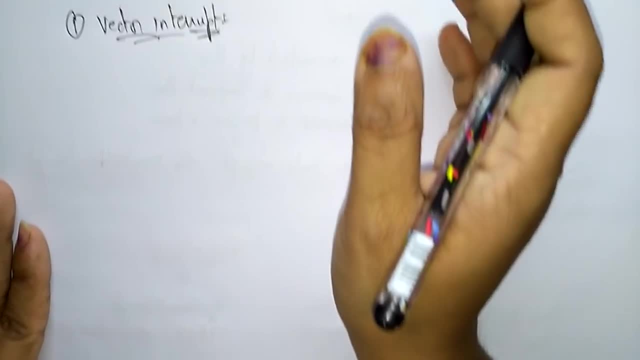 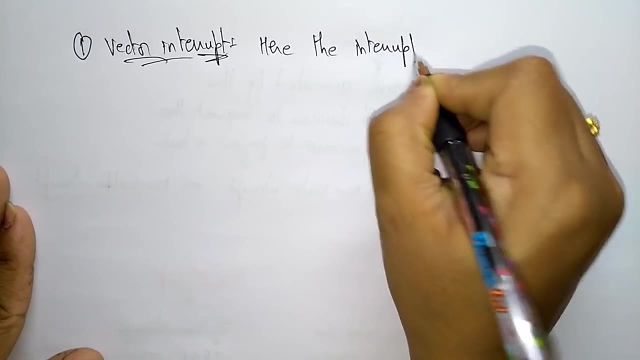 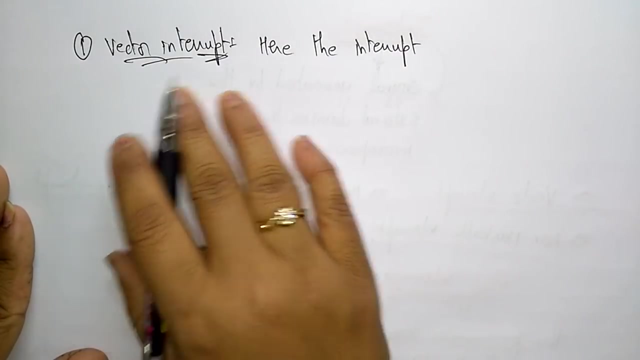 so whenever the interrupt address is known to the processor then you call it as a vector interrupt. here the interrupt address means from where the interrupt is coming, from which device the interrupt is coming. that will be known by the processor that you call it as a vector interrupt, here the interrupt address. 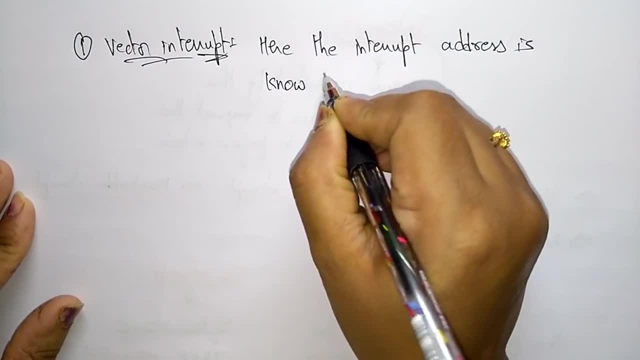 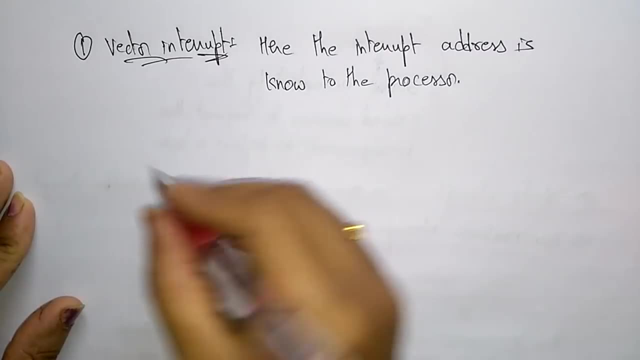 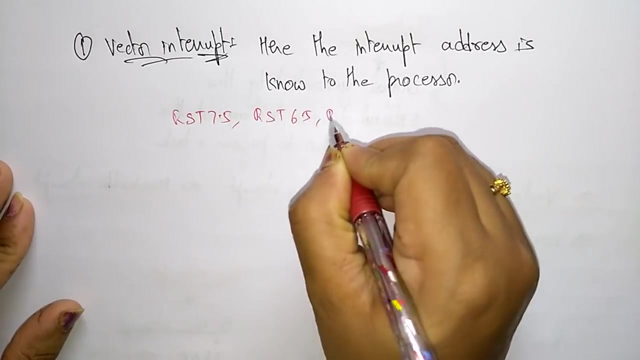 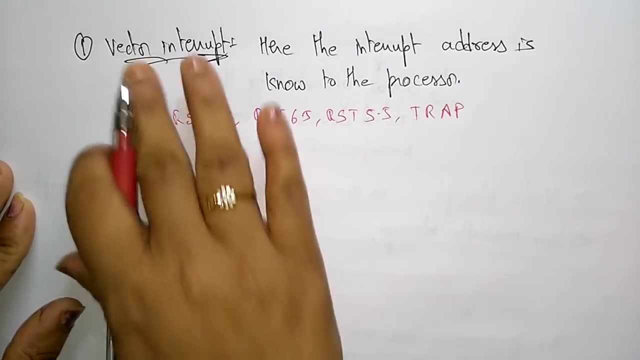 is known to the processor. so these interrupts can be generated with the signals uh pins like rst 7.5, rst 6.5, rst 5.5 and trap. so with the help of these pins the vector interrupt will be generated. so uh, when a vector 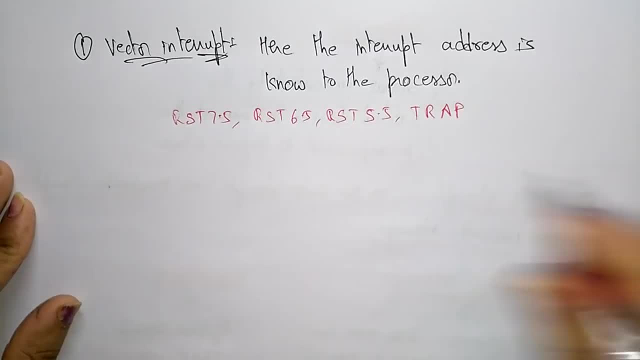 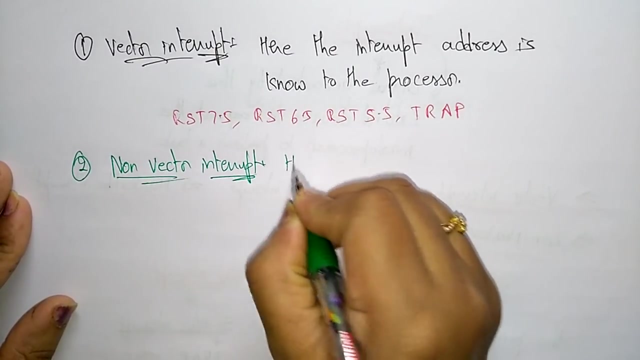 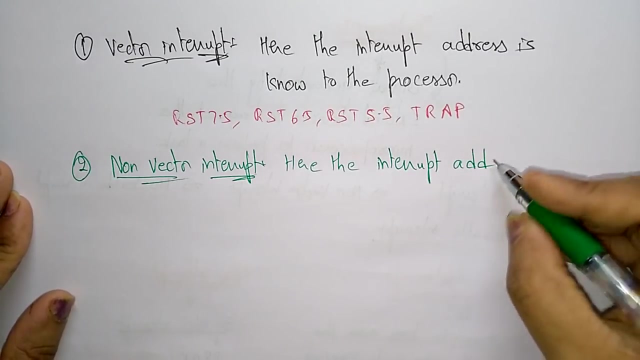 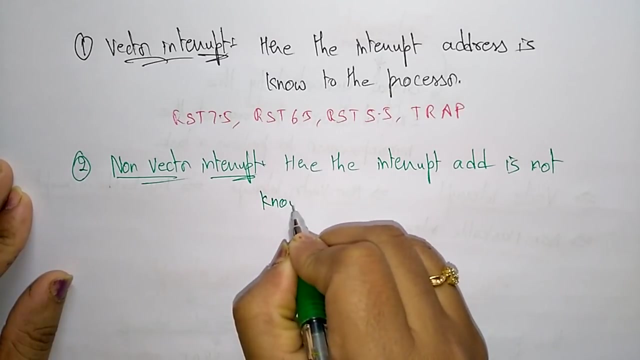 interrupt means the interrupt address is known to the processor with the help of these pins. now coming to the next step. so next is vector interrupt. so non vector means the address will not known to the processor. so here the interrupt address, interrupt address, is not known to, not known to the 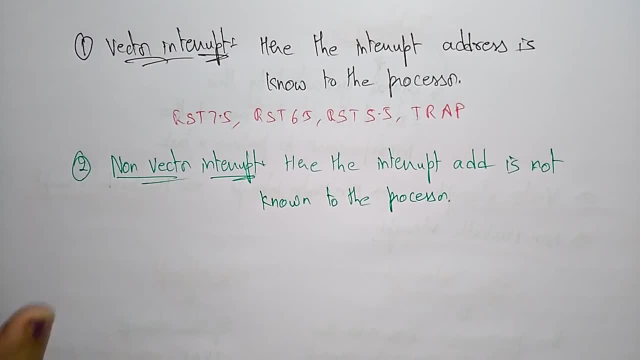 processor. so interrupt address. uh needs to send externally by the device to perform interrupt. so only there with the help of the external device. only it accepts. the processor knows the. this is the address of the interrupt, from where the interrupt is coming. so the example for this uh non vector interrupt is: 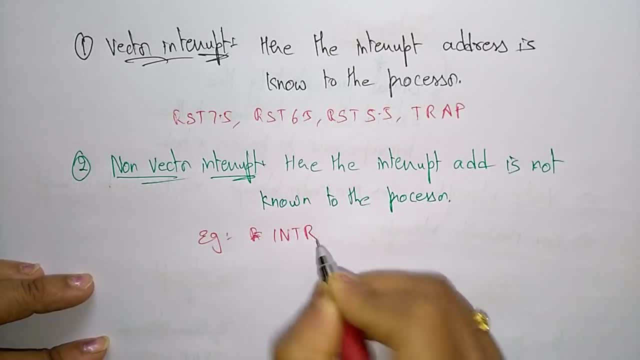 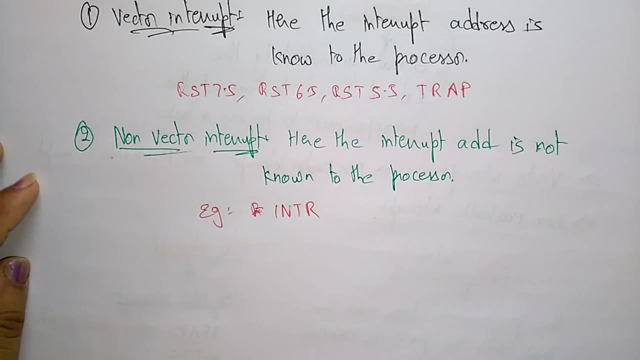 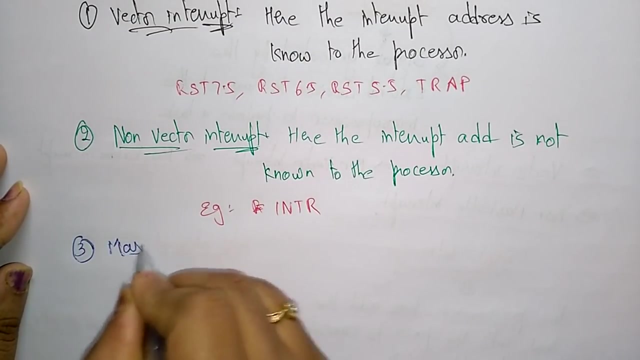 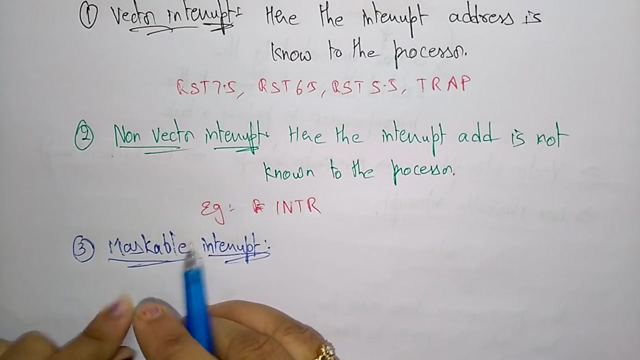 intr. intr. interrupt is nothing, but it is a non vector interrupt. now coming to the third one. so what is the third one here? maskable interrupt, maskable interrupt. so what is this maskable interrupt? he, in this type we can disable the interrupt. maskable. the name is saying we are masking the interrupts, just. 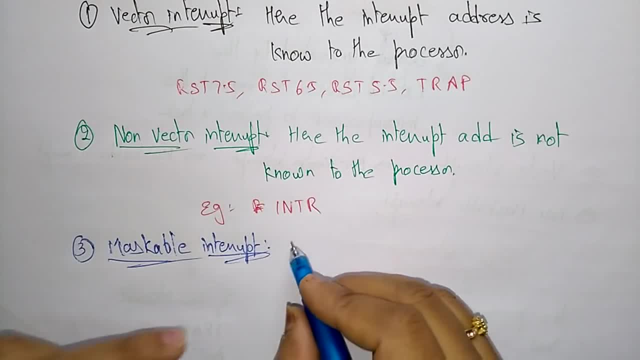 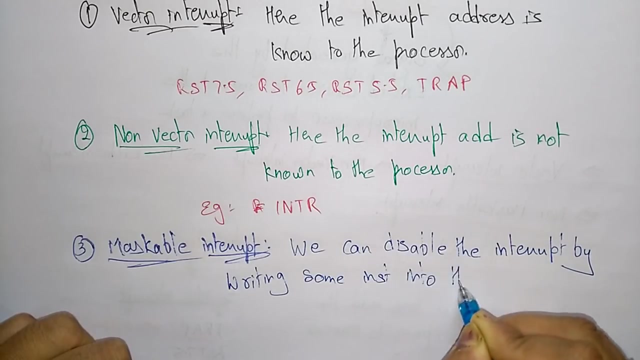 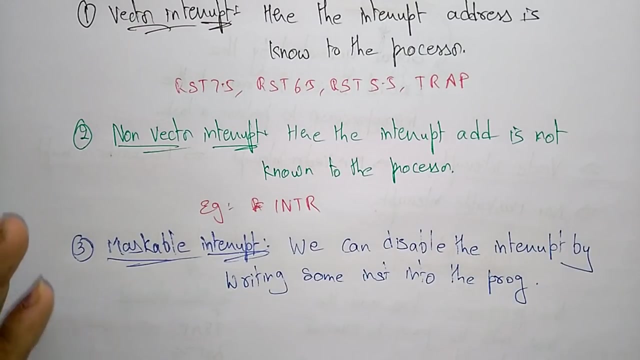 it's not appearing means maskable here. in this type we can disable. we can disable the interrupt by writing some instructions into the program. so we can disable enter by writing some instructions into the program that you call it as a maskable interrupts. the examples for this maskable interrupts: 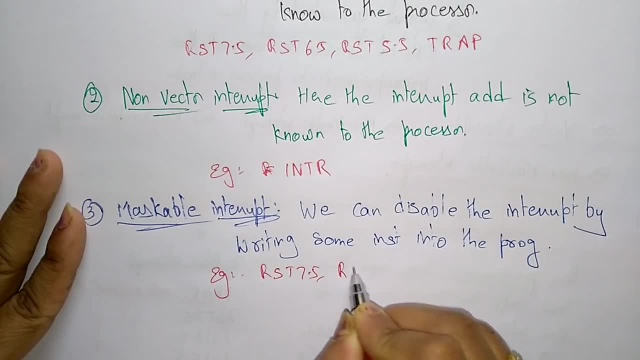 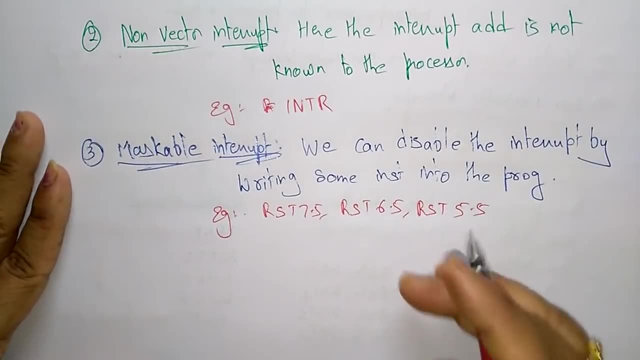 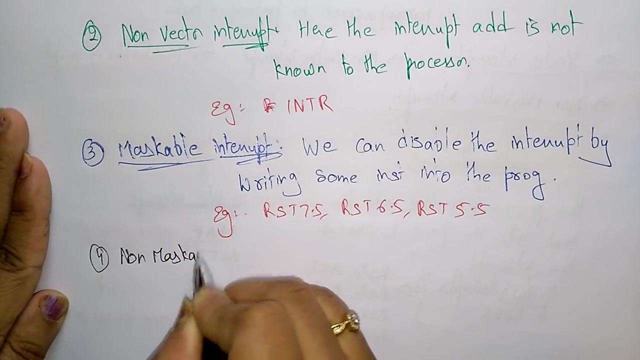 is rst 7.5, rst 6.5, rst 5.5. so these are the maskable interrupts. and coming to the last one, what is that? that is, non maskable interrupts means those are not disabled. non maskable interrupt is rst 7.5. but thinking it as a maskable interrupts means they are not necessarily. 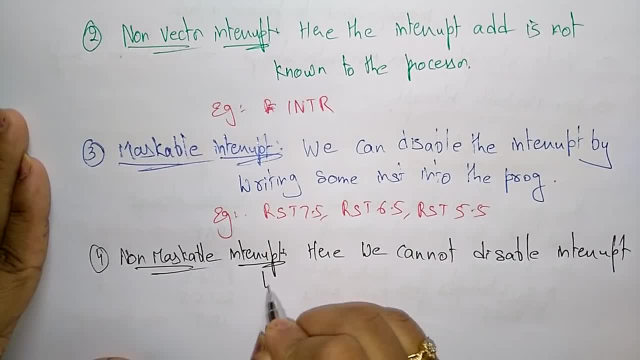 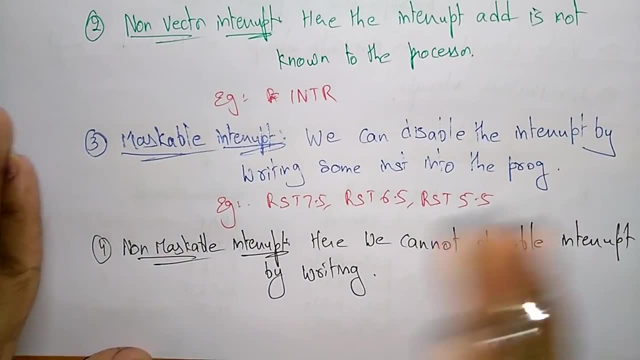 we cannot disable interject by writing. so what does this make sense? even if they are belongs or you can not, disables are not the exact same for any Angular. we can not remove the text as we are not using als or with them. so it means if we try to input the text again and once we 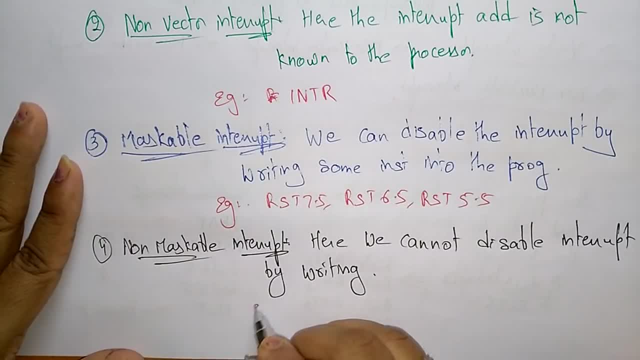 pass through the text, it will switch back to the otheryll Reg Russell, I not itself box is said to mean no and non maskable. what does that mean now? what does that say now, here we cannot say except déne, here we cannot disable. interrupt by writing. so here we cannot disable. 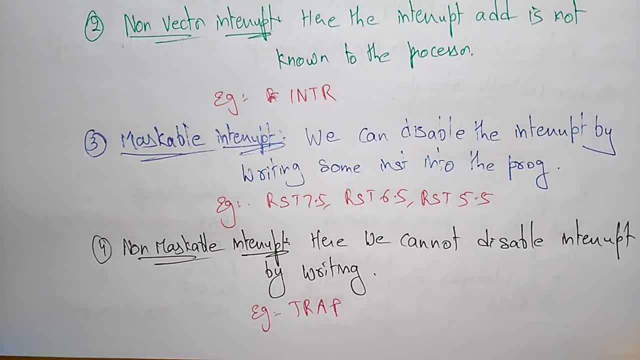 interrupts, interrupt by writing. so only some instructions into the program. here we cannot disable by writing some instructions into the program. so the examples are: nonуки Bay, little adult conversations. the processor has to stop that present work and it has to take the trap signal request and it the